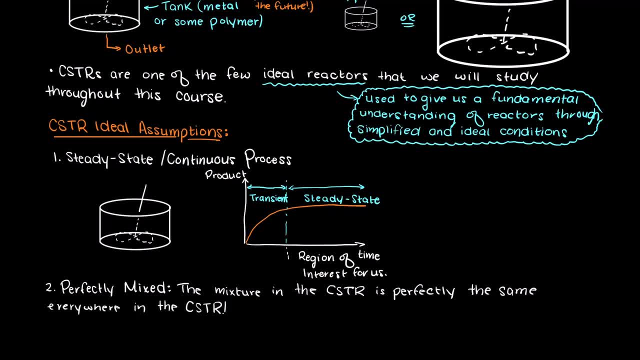 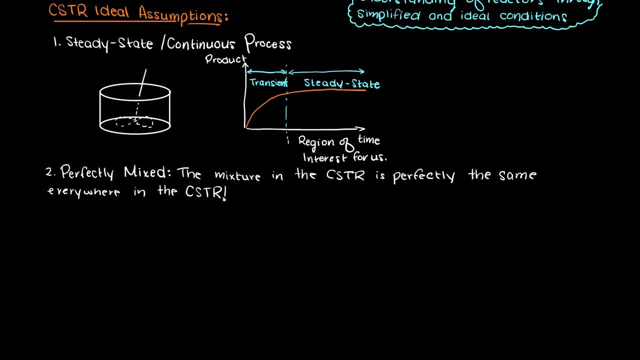 This means that the mixture within the CSTR is so well mixed that the composition, temperature and other characteristics of the mass anywhere within this reactor will give us the same results. So because our CSTR is a steady state reactor, that means that when operating we will continuously 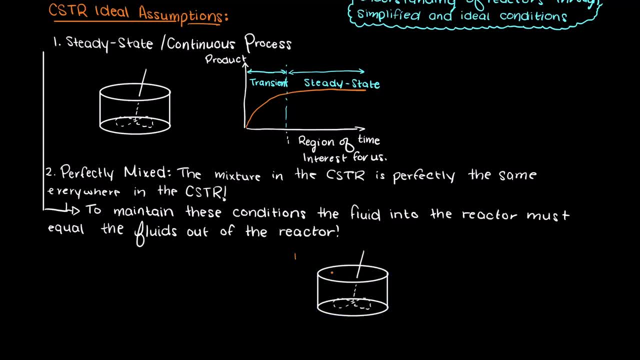 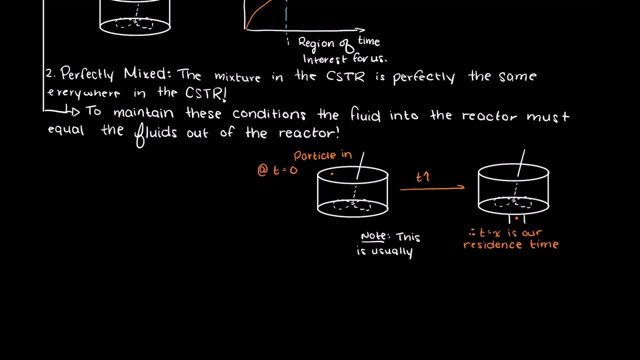 be feeding it reactants and removing the products at the same rate, The idea here being that the new reactants enter our tank, stay for a certain time period. this is called a residence time- how long a particular particle will stay within our reactor and then leave our reactor once the 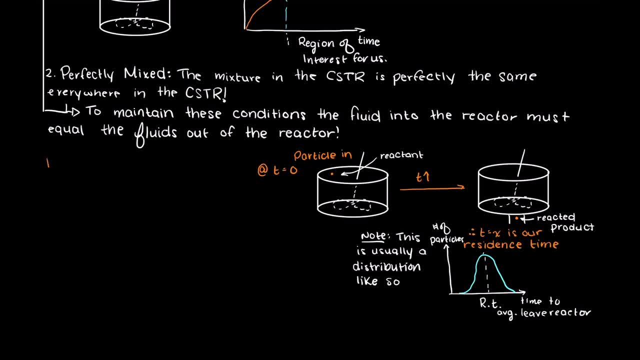 reactant has become a product. Some advantages to CSTRs are that they give us a lot of control over the components within our reactor, such as the temperature. They are relatively simple and therefore less likely to break down. Additionally, they have lower labor costs as 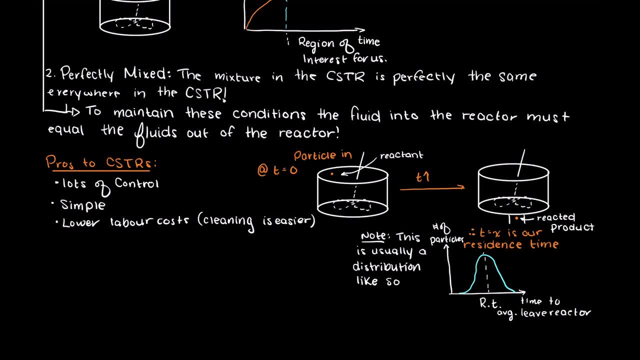 cleaning the machine and running them are both easier compared to more complex reactors. Our control over things like the temperature are due to the perfectly mixed assumption that I mentioned earlier. If we had a heating or cooling jacket over our CSTR, the energy is obviously. 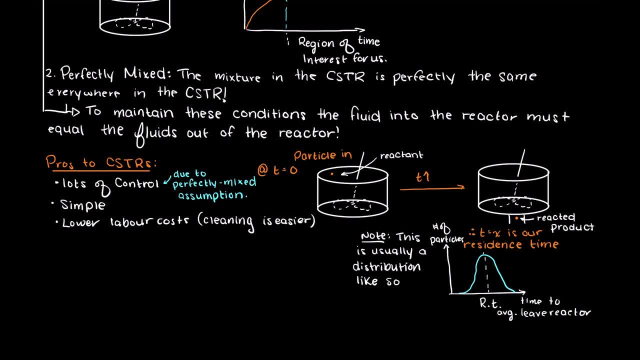 going to be applied to the walls of the reactor. However, since the temperature is so high, the convection of heat is quickly going to reach a steady state. Therefore, we have excellent heat transfer occurring Additionally. CSTRs are great as they are both simple and cost effective. 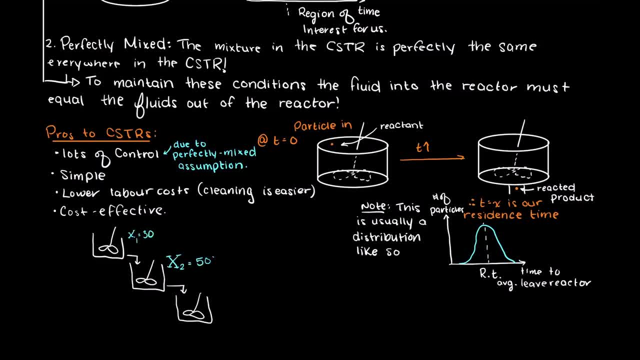 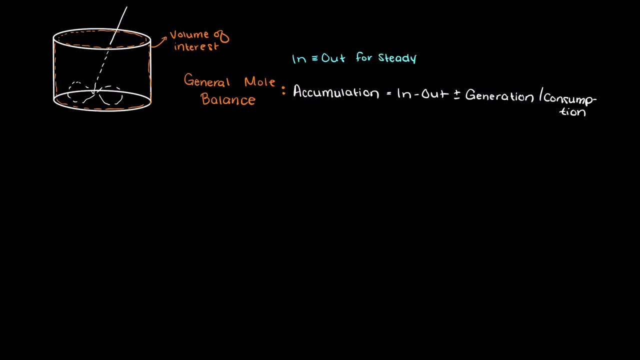 efficient in the process. They are not very efficient in the process. They are not very, otherwise we would not have a steady state right? So this means that our accumulation term will be zero, and this will always be the case for a steady state system. So we just have the moles. 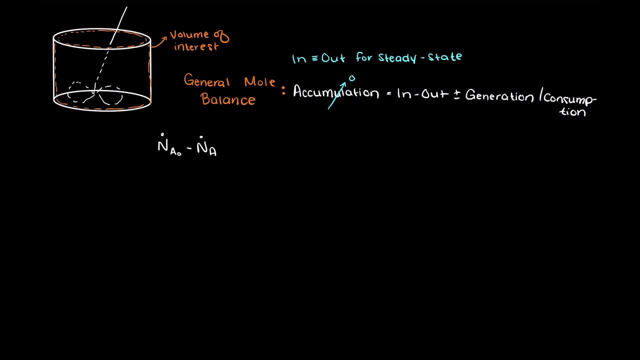 of component A coming into our system, minus the moles of component A leaving our system, plus the amount of moles generated within our reactor. This generation term here could also be the consumption of A, or both, depending on what part our component A plays in the reactions.